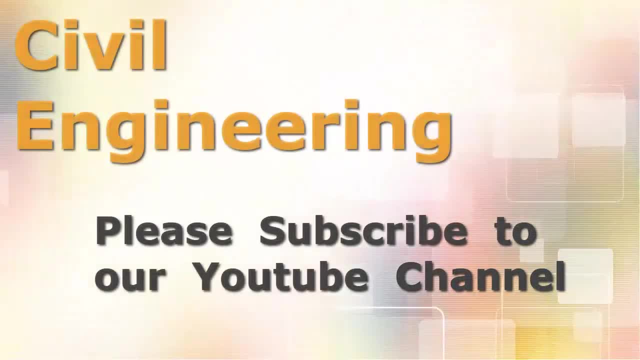 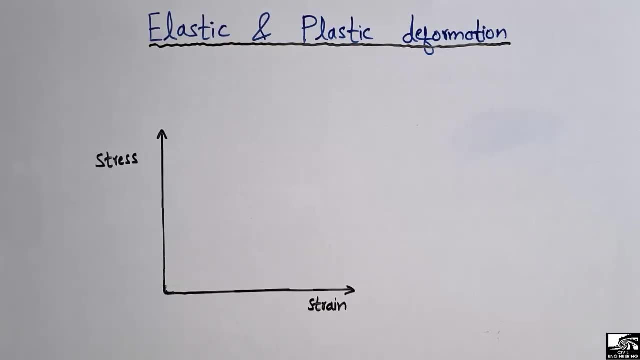 Hello guys, welcome back to the Civil Engineering YouTube channel. Please subscribe our channel for daily civil engineering videos. Today's our lecture is about the difference between the elastic and plastic deformation, So I would like to explain the main difference between these two types of deformation with the help of the example. So let's consider. 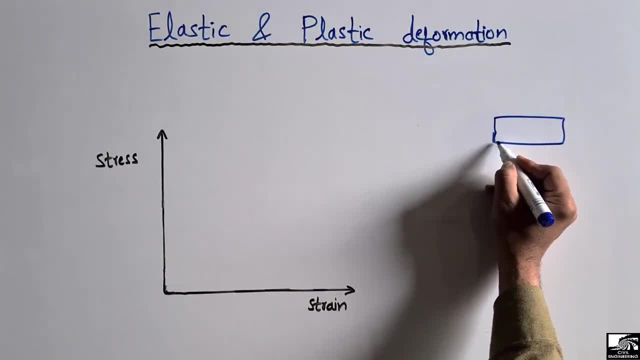 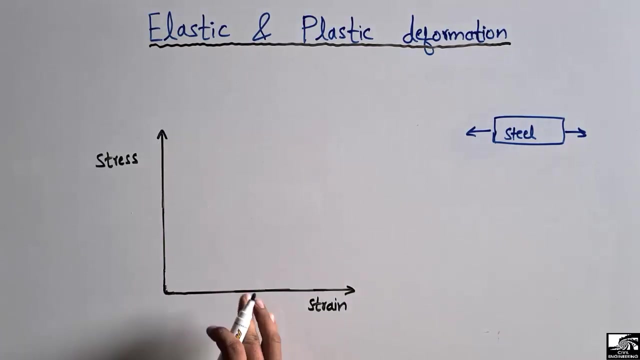 that we have a steel material here. This is a steel material and I applied the load on both sides of this steel material. So there will be some stresses and strain created inside this steel material. So we can see here the stress and strain curve on the left side. 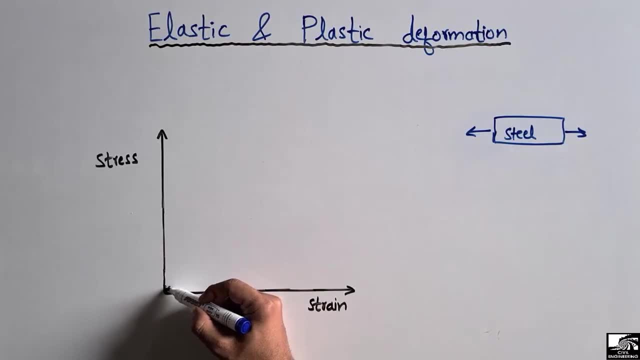 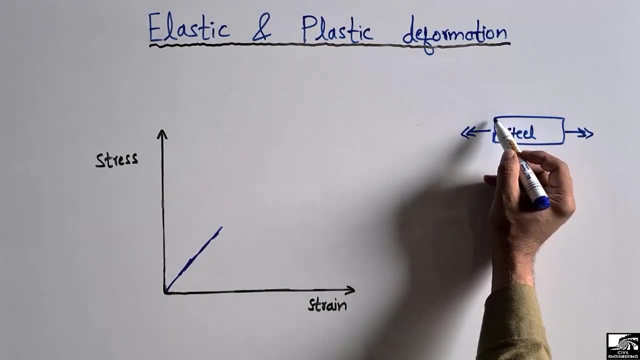 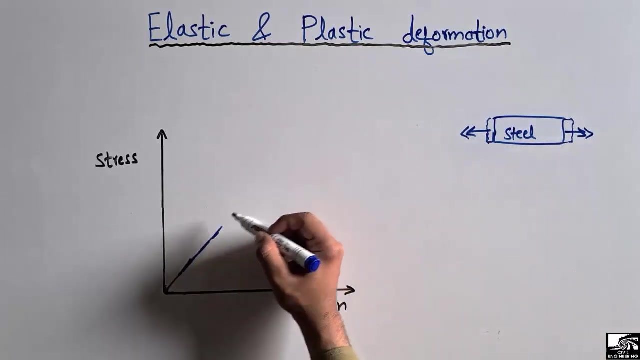 So by applying the load on the steel material there will be some stresses and strain created inside this material And by increasing the load on this material the material will tend to deform and expand. So it will expand to this position. And by increasing the load 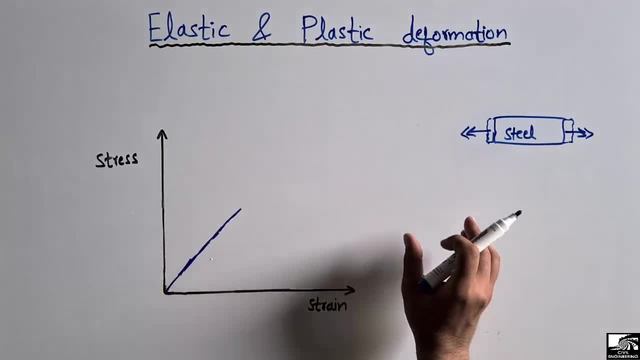 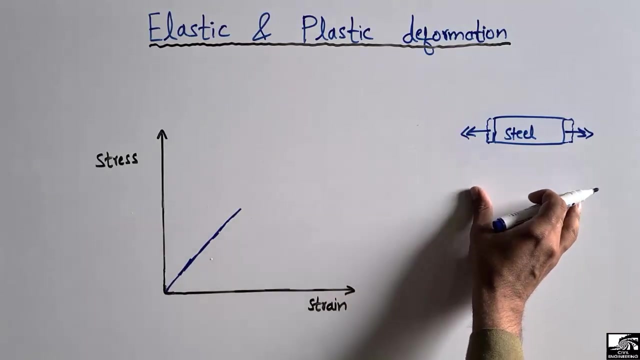 on this material, the stress and strain will increase. So now, if I remove this load, the material will come back to its original position. So the point where I remove the load and the material again comes to its original position, this deformation is known as the elastic deformation. 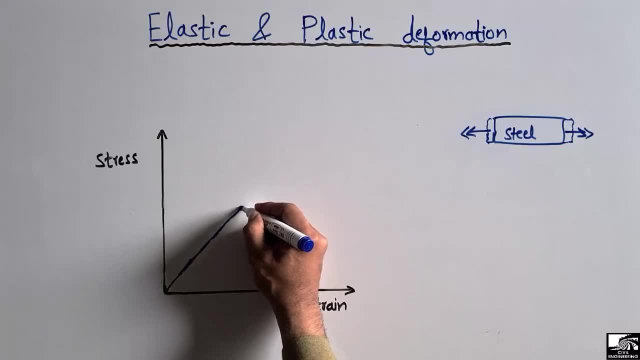 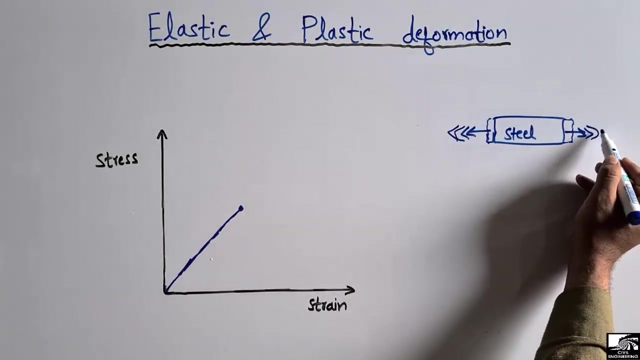 of the material. So I will consider that this point up to this point the material can come back to its original position after removing the load. So we remove the load on this material and it will improve the deformation and the material will move back to its original position And I will see the stress and strain curve on. 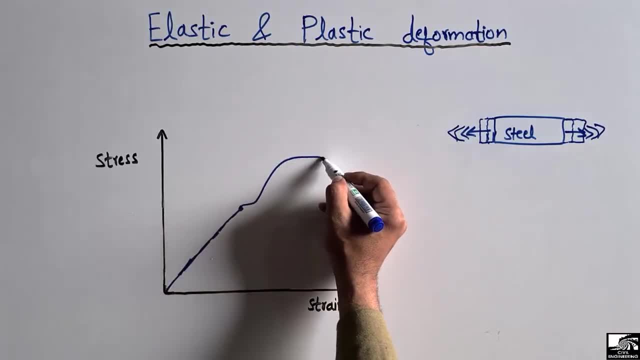 both sides of this material. The bottom of this material will be shown as the elastic deformation of the material. And now, if I increase the load, the material will tend to increase and expand And also there will be some stresses and strain increase in both. 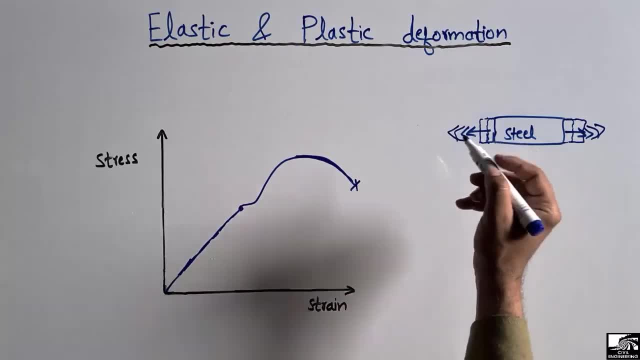 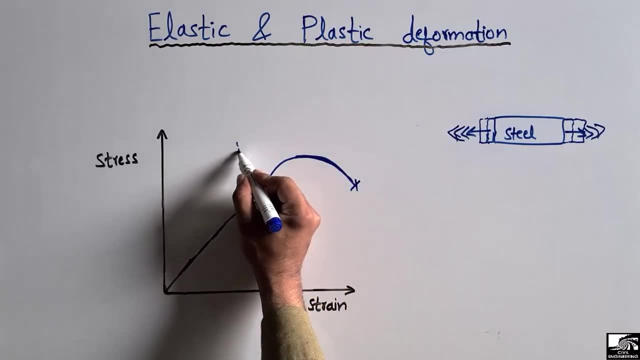 the directions until the material is fractured here. So this is the general stress and strain. remove this load, the material will not come to its original position. so this was the stage, so this was the main line between these two types of the deformation. up to this point, up to this load, the material was able to come to.